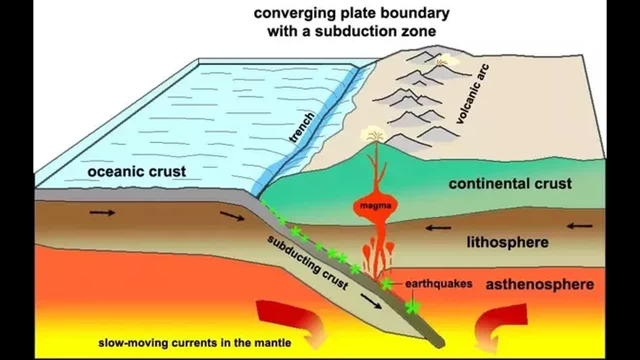 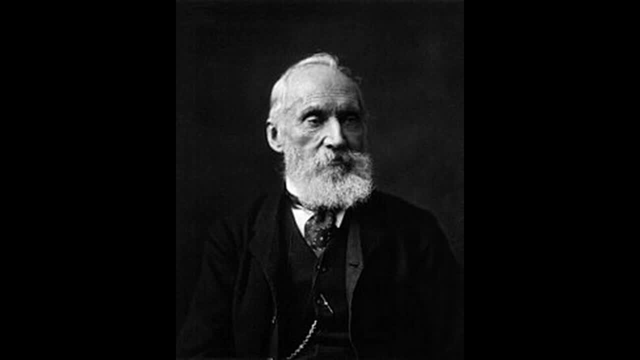 substance which acts as a fluid for the mantle to flow through. So if we were to imagine a fluid over vast time spans, In 1862, Lord Kelvin estimated the age of the earth to be roughly between 20 million and 400 million years old. He did this by calculating how long it would take. 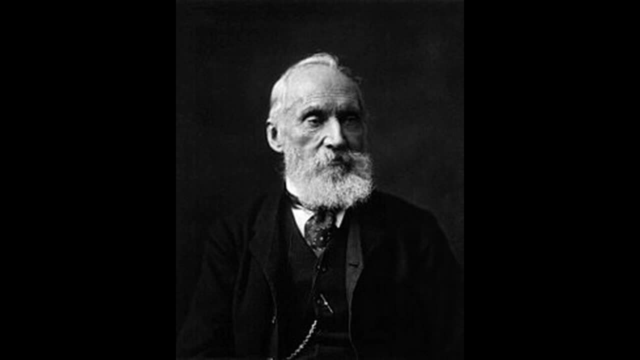 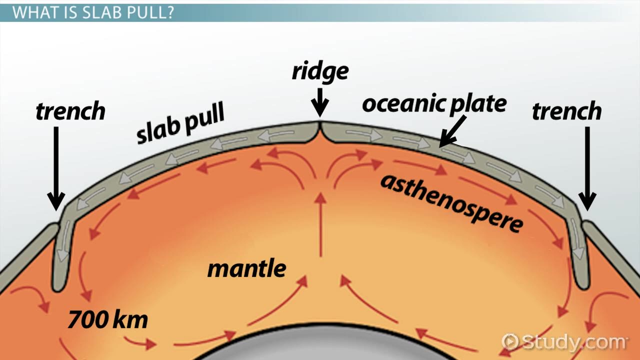 for the earth to cool down from a molten object to its current state. using his understanding of thermodynamics, However, Kelvin didn't take the heat that was produced by radioactive decay into account, nor how convection within the mantle maintains a high temperature gradient inside the 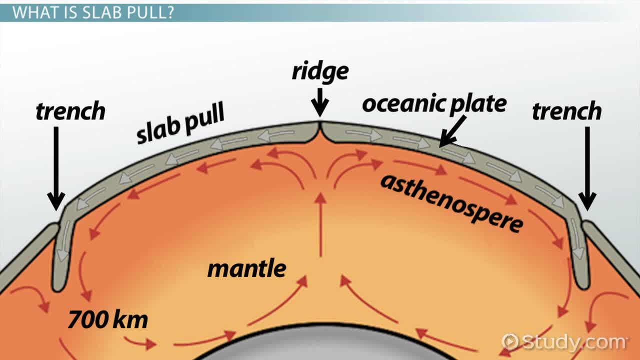 crust, both of which push the mantle to a higher temperature gradient. So if we were to imagine a fluid over vast time spans? In 1862, Lord Kelvin estimated the age of the earth to be roughly between 20 million and 400 million years old. He did this by calculating how long it would take for 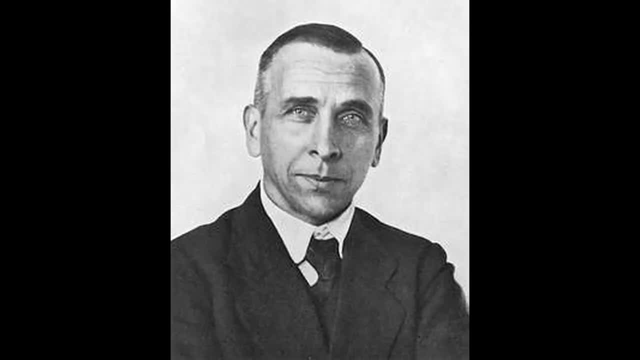 the earth to cool down from a molten object to its current state using his understanding of thermodynamics. Although you couldn't blame Kelvin for not knowing these things, not even Alfred Wegner, the one who spearheaded the theory of plate tectonics in the early 20th century. 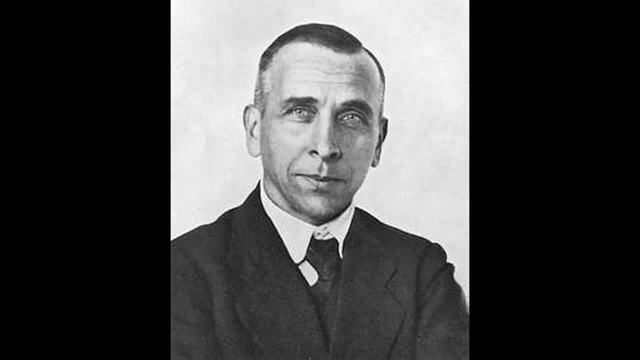 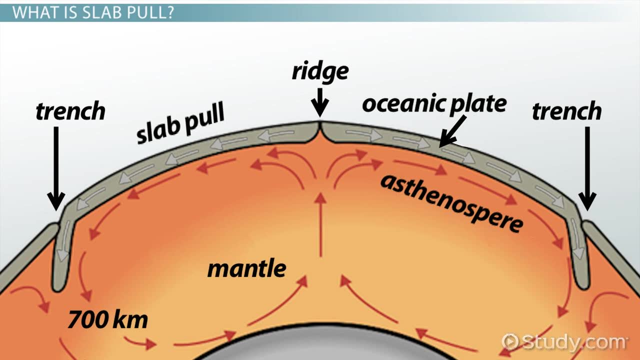 took convection into account. Wegner was subject to ridicule, since most scientists at the time could not see how it was possible for the continents to plow their way over the oceanic crust. Now we know that the continents move by friction between the solid lithosphere above. 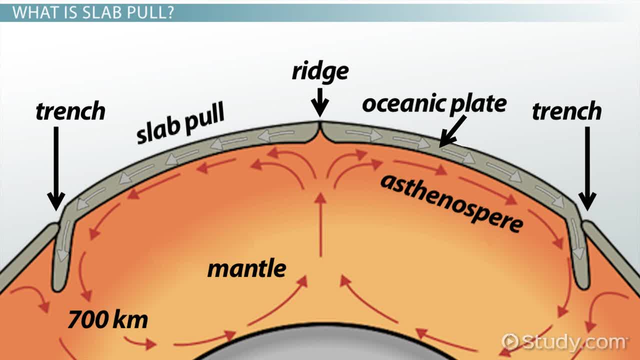 and the convection currents in the asthenosphere below, and that the convection currents inside the mantle are not as strong as they used to be. So we know that the continents move by friction, in turn, driven by the heat from the earth's core. The precise physics of these currents are still. 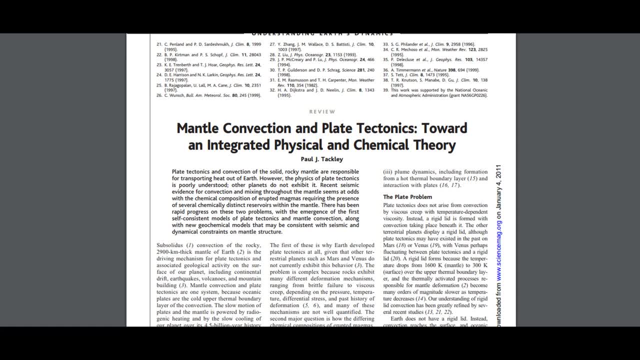 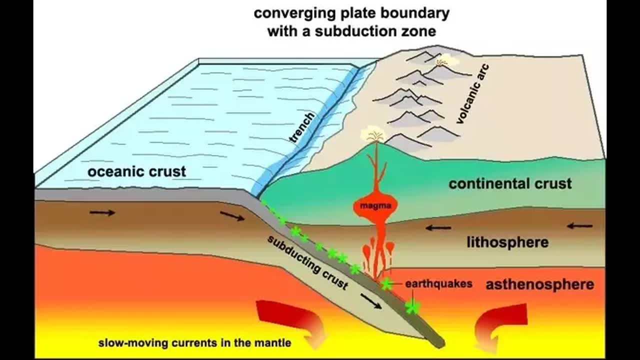 being studied by researchers, though, as described by the 2000 paper Mantle Convection and Plate Tectonics Towards an Integrated Physical and Chemical Theory. Anyway, there is a limited amount of space on earth, so plates are bound to bump into each other One way. they do this. 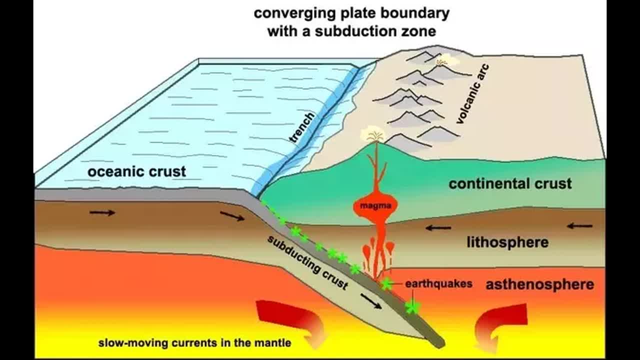 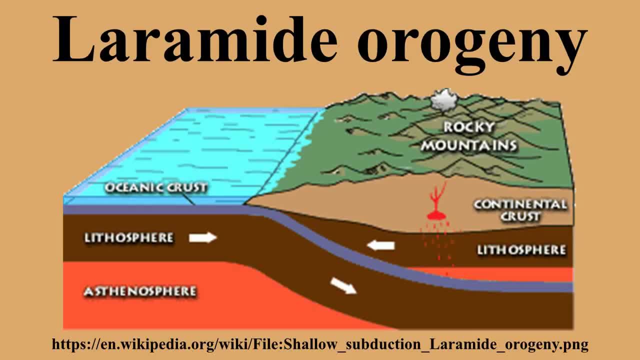 the pertinent way is at a convergent boundary. The collision of two plates has a number of results, including earthquakes, volcanoes and orogeny, among other things. Of these, we're after orogeny, which is defined as a process in 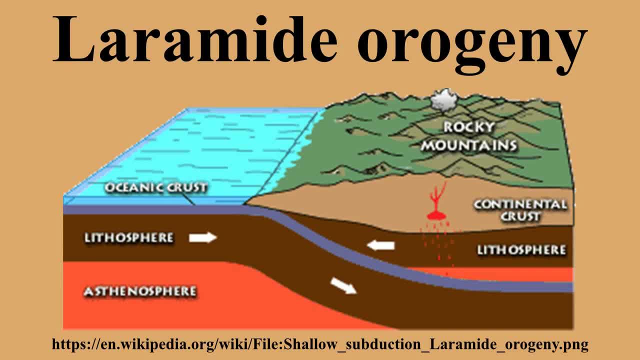 which a section of the earth's crust is folded and deformed by lateral compression. Importantly, mountains are formed during this process. The plates collide and the less dense plate is pushed up. Meanwhile the denser plate is pushed under, called subduction, where it is to be recycled.